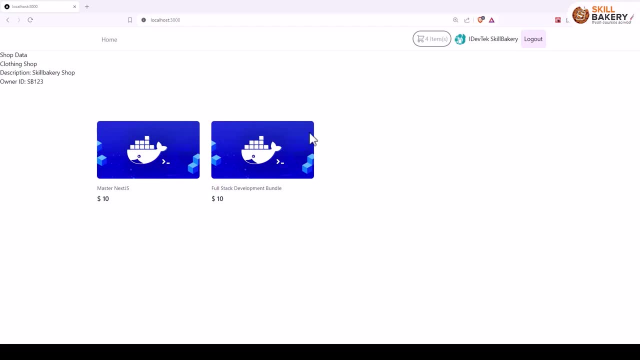 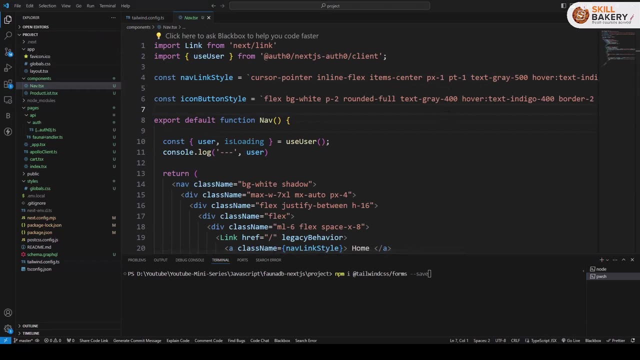 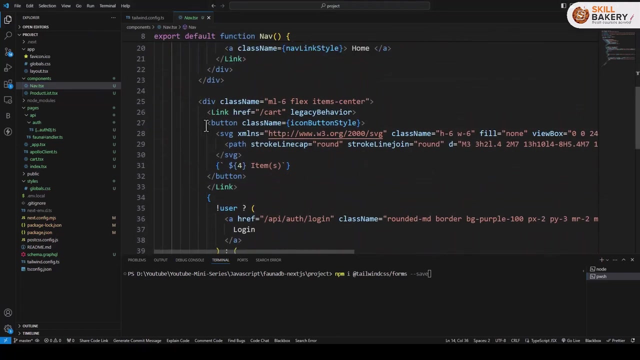 able to add new shops. So the first thing that we need to do is in our nav component. so here in our navtsx file, we'll be first of all adding a menu option called manage shops. So here you can see, we have our cart and then, once the user is logged in, we are showing the name of the logged 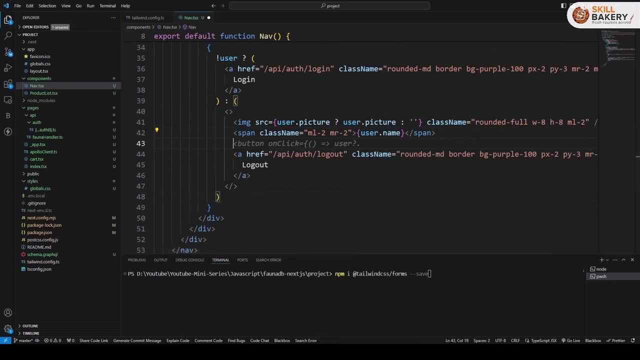 in user and just after that we'll be introducing this new menu option called manage shops. So here we'll have our manage shops option coming up and here you can see that it's reflecting now in the page. but as of now we don't have this page called manage shops. So what we? 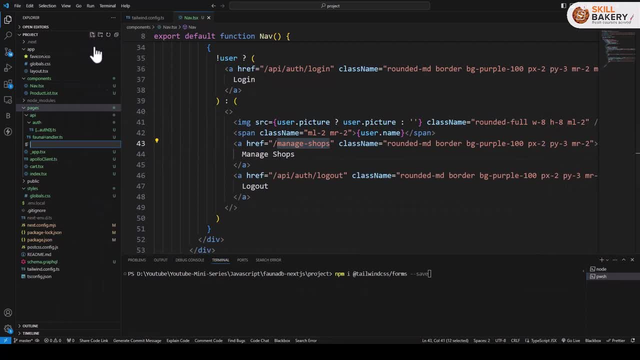 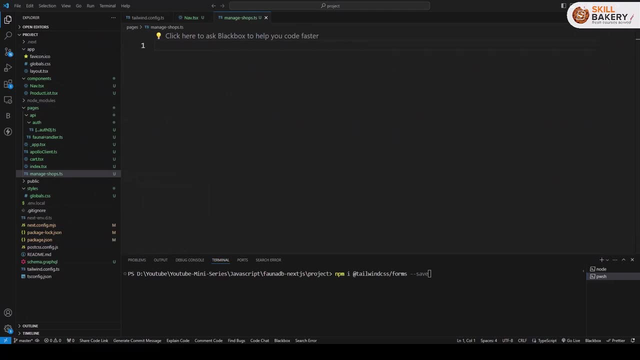 need to do is under pages we need to create one. So we'll say manage shops and inside this we'll be writing our manage shopstsx extension, and here you'll notice that we are calling this form a new shop form which is being rendered over here. 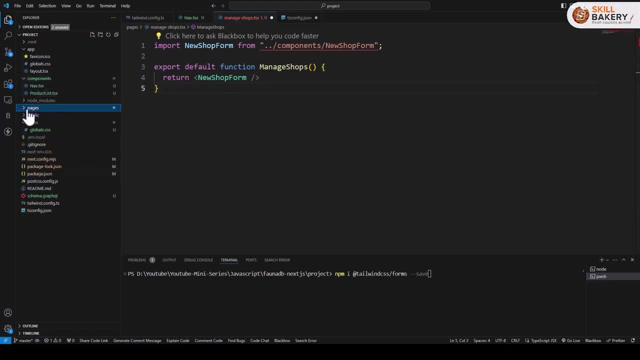 So the new shop form is going to be a component and it will be created inside this components folder, So let's go ahead and do that. We'll be calling it as new shop formtsx and inside this, first of all, we'll go ahead and import a couple of things like user state from react and we'll 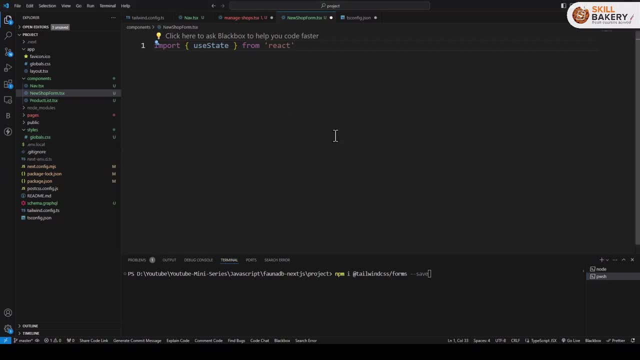 then have our form created. So we'll say const- new form shop, and within this we'll be going ahead and we'll be creating the form data. So here we have name, description and cover image. These are the three things that we'll be asking the user to provide, and we'll then have the handle change event, which 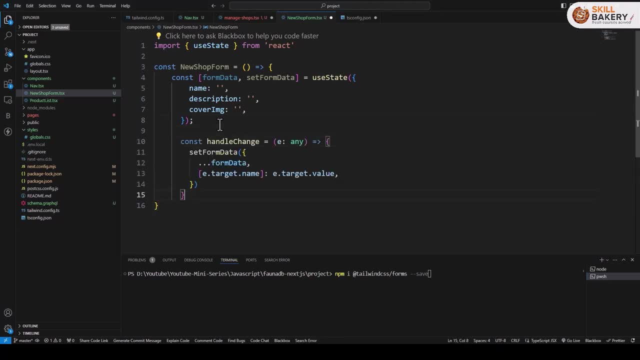 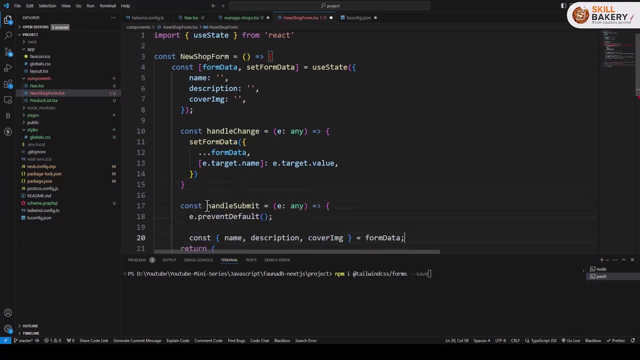 is going to set the value of these form fields once the user is entering it, and after this we'll have this return statement. So here we are, creating the form. So now we'll just type in this new form. I'm going to double click on this and we'll be doing a couple of things. 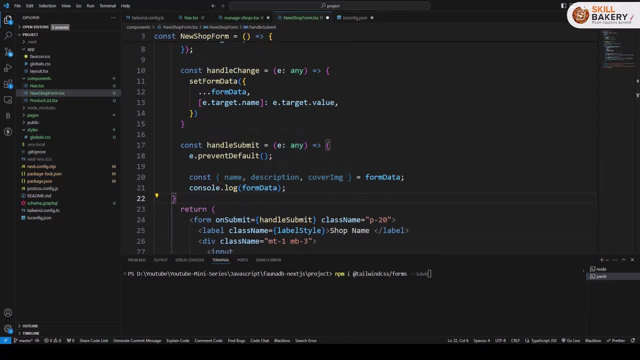 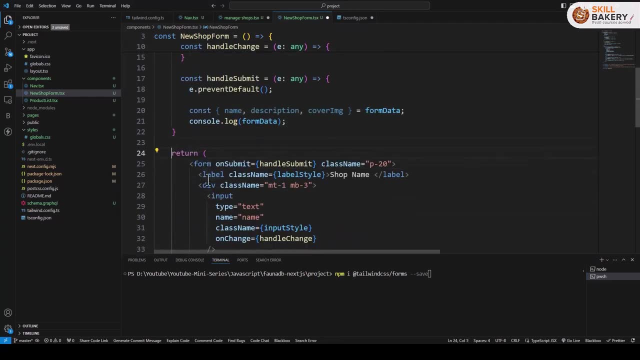 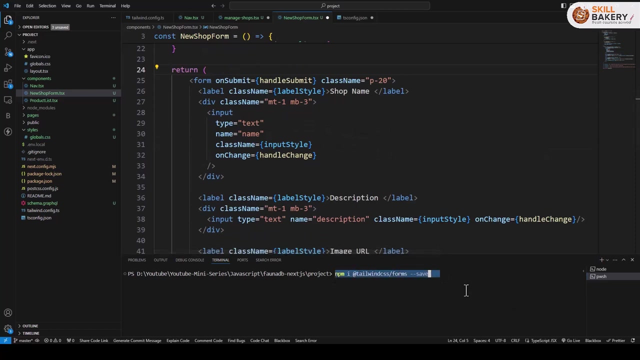 So we'll just type in some button styles and form elements So we'll also have the handle submit implementation. So for now we'll be just having this form data thing and we'll be just logging it in the console And here we are creating the form.